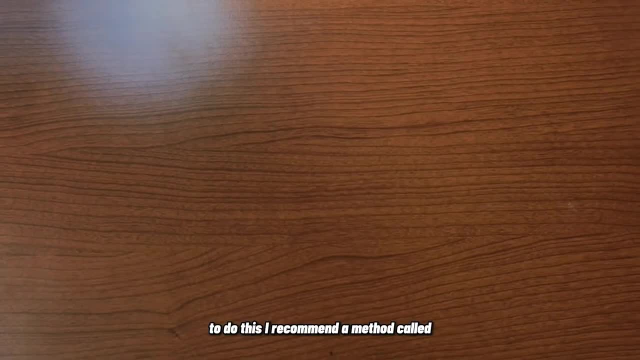 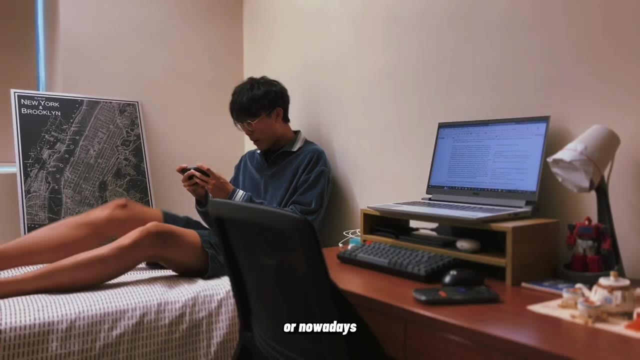 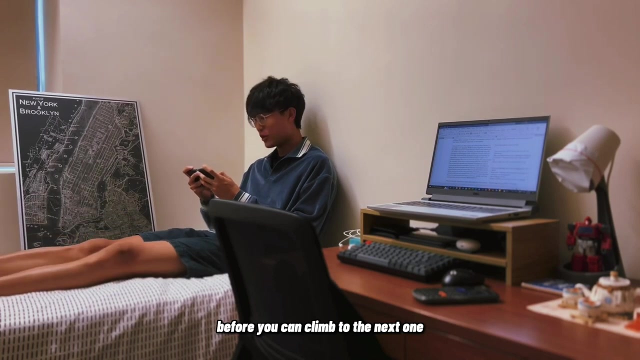 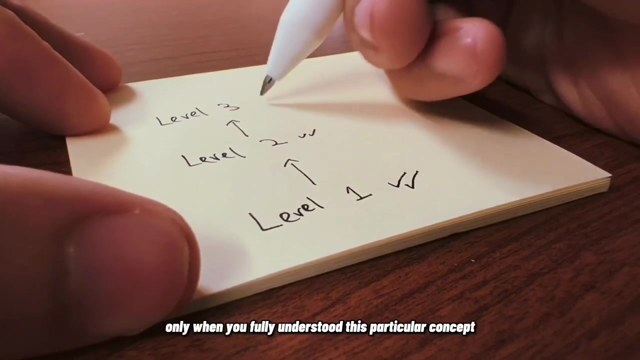 one of these LOs or concepts. To do this, I recommend a method called the game checkpoint approach. Let me explain. You see, when you play a game, be it first-person shooters or, nowadays, online games like Minecraft, you do not have the need to. 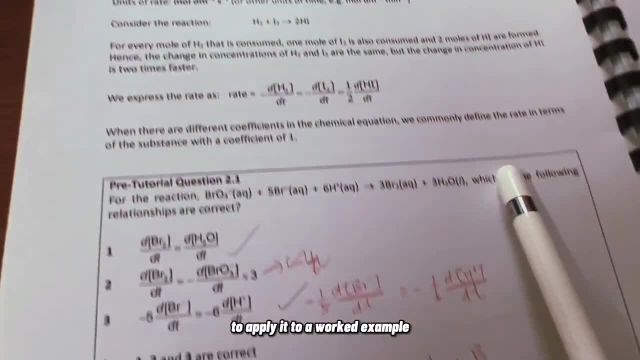 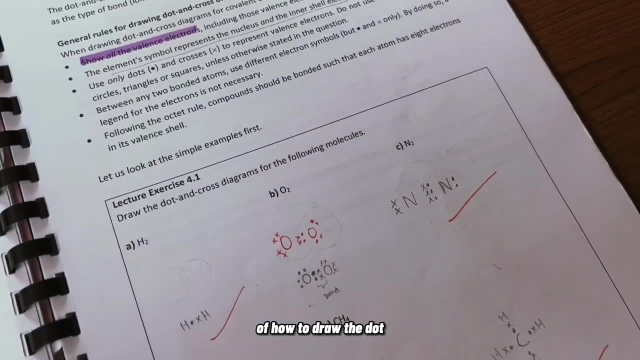 know the correct turn tables or ranks that you need to clear before you can climb to the next one. Similarly, you should also learn the concepts in chronological order, one by one, So only when you have fully understood this particular concept, its meaning, its applications or even how to use this. concept to apply it to a work example, then can you move on to learn the next concept, For example, when you're just learning about the concept of how to draw the dot and cross diagrams of polyatomic ions or solving back titration calculation questions. make sure, this is a very useful lesson for you. 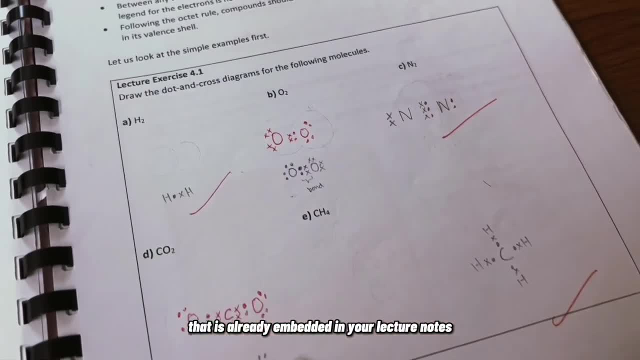 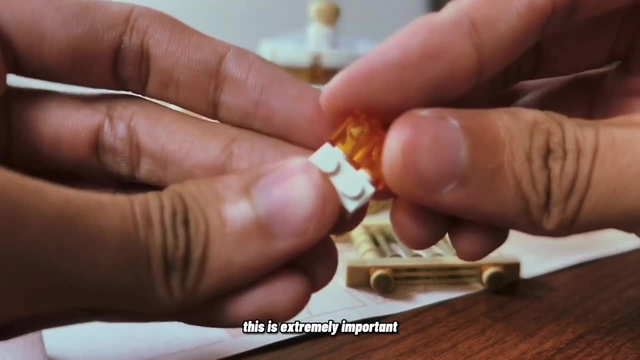 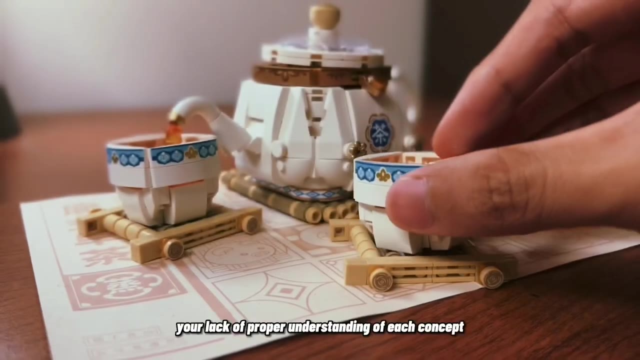 that you utilize the work examples that is already embedded in your lecture notes and ensure that you get all of them correct before moving on to learn the next thing. This is extremely important as, more often than not, each concept links to the previous one in one way or another, and if you fail to do this, your lack of proper understanding. 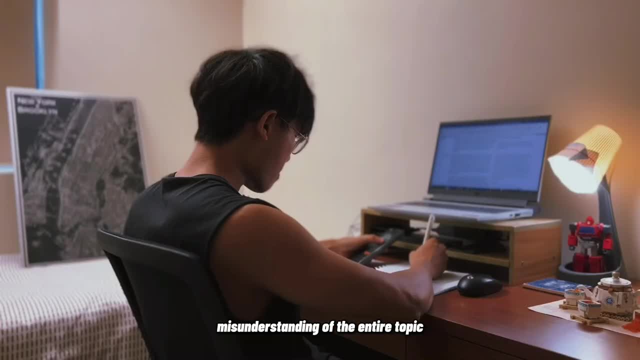 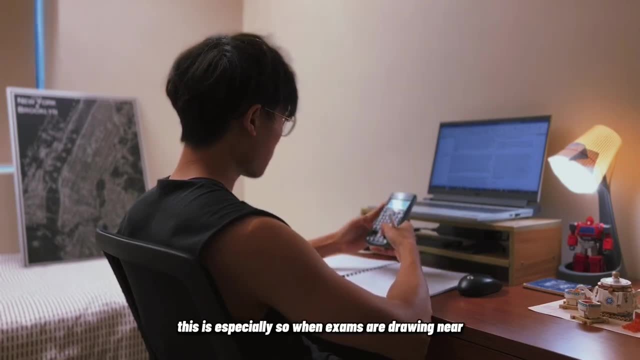 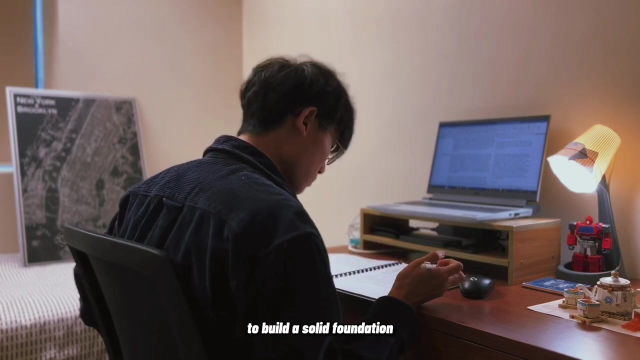 of each concept will snowball into a huge misunderstanding of the entire topic, which will only serve to bring in more stress and more chaos into your life. This is especially so when exams are drawing near, because you will highly likely find that you have forgotten most of what you have already studied because you did not do the work to 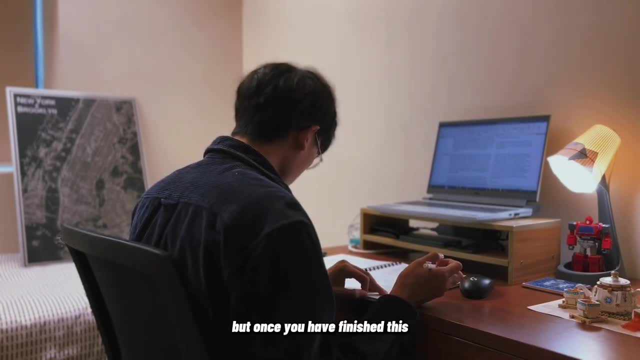 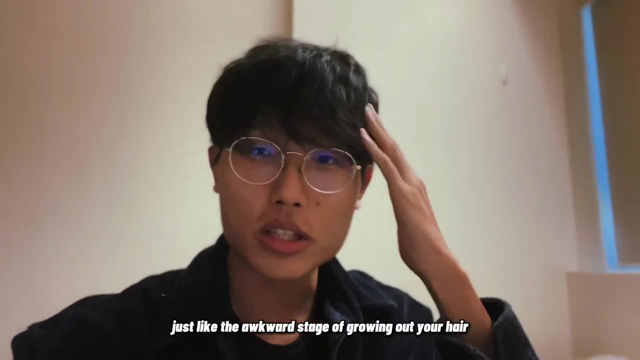 build a solid foundation. But once you have finished this, you can now level up and enter into the next stage of your learning curve. Now I like to think of the intermediate stage, just like the awkward stage of growing out your hair, because you are sandwiched in between being a complete noob and being an exam-ready. 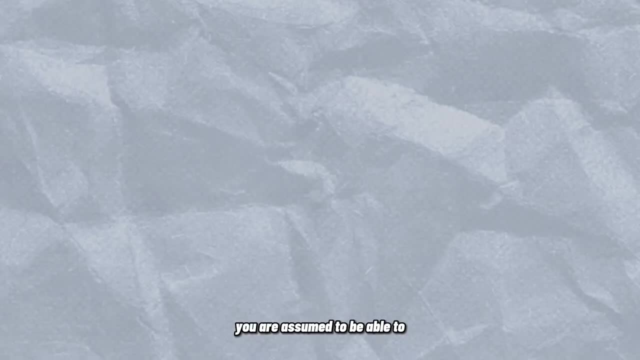 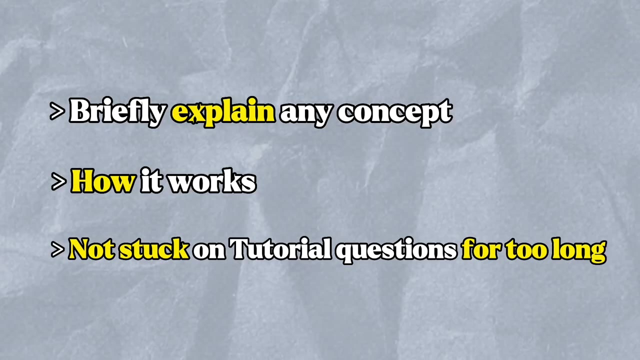 academic weapon. In this stage, you are assumed to be able to briefly explain to me any concept that you have or how it works, and able to do your tutorial questions without being stuck for too long. What you are lacking- which is also what we should be emphasising on- is practice, practice. 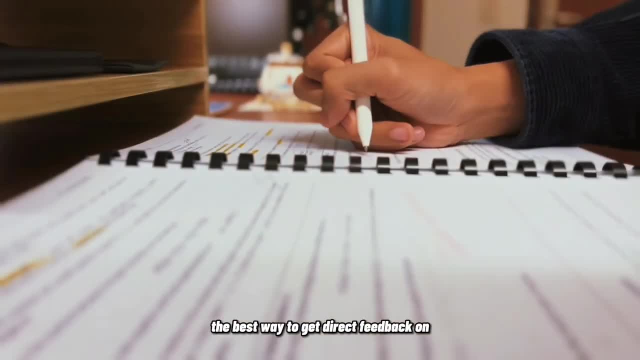 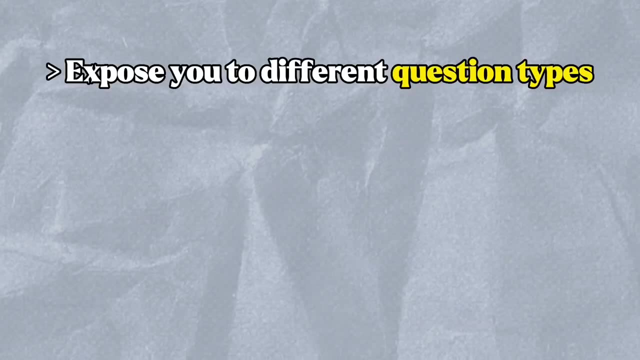 and more practice. Doing questions is arguably the best way to get direct feedback on how much you have understood a concept and how well you can apply them, And doing more of these can expose you to the type of questions that usually come out and how they are phrased, and if they ask this in a certain way, you will know exactly what. 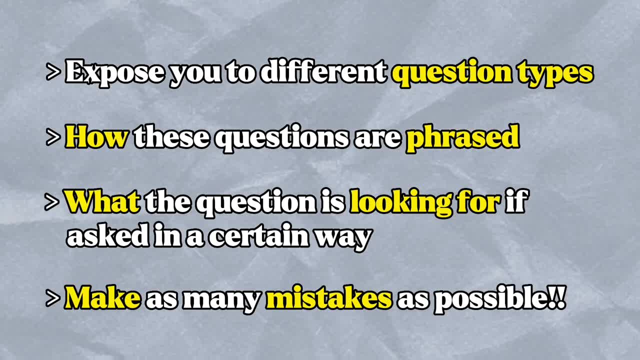 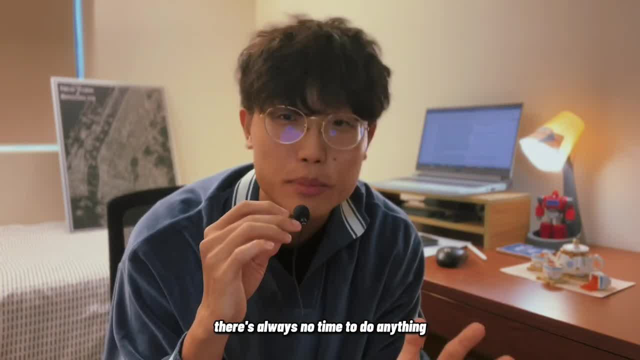 they are looking out for. So if you have any questions, feel free to leave them in the comment section below. Now, I've been in your shoes before, so I completely understand that there's always no time to do anything. but many doesn't have to be 100 questions, it doesn't even need. 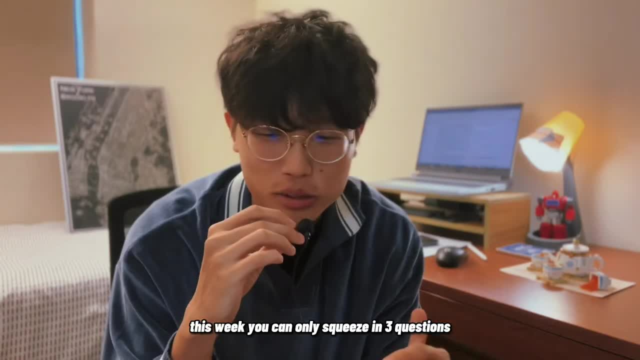 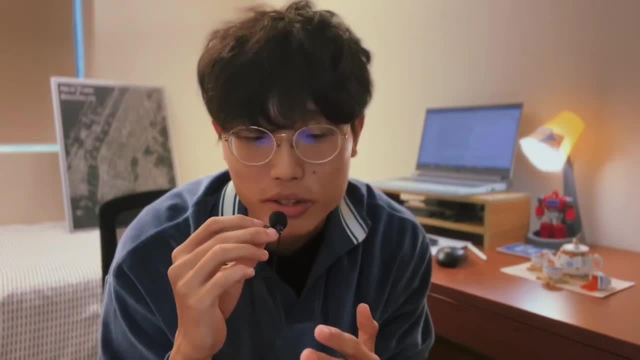 to be 10 questions. If, for whatever reason, this week you can only squeeze in 3 questions, I actually think that it is very commendable. I am all for celebrating progress over perfection. You see, everyone is now obsessed about results, but everything you want to succeed as a student. 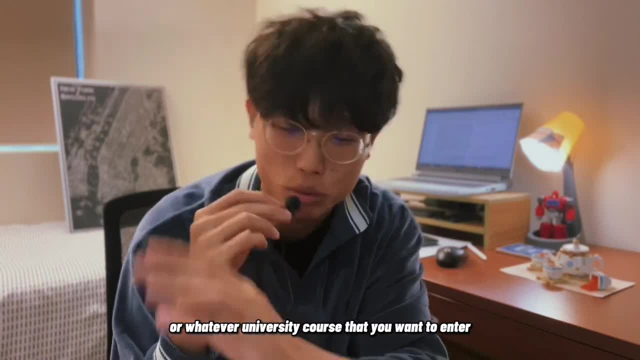 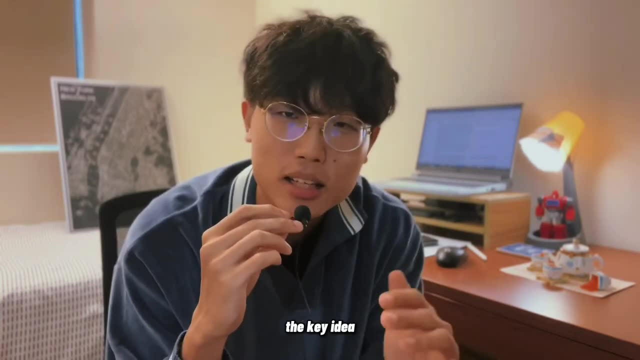 whatever rank points that you want to get or whatever university course that you want to enter, all comes down to not obsessing about the results, but obsessing about your own progress. The key idea that I want to drill into your head today is to be consistent, so that you 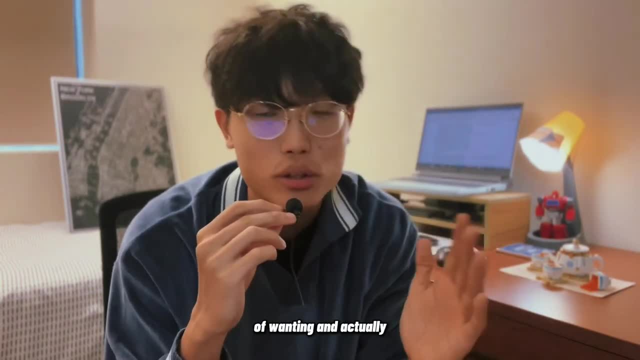 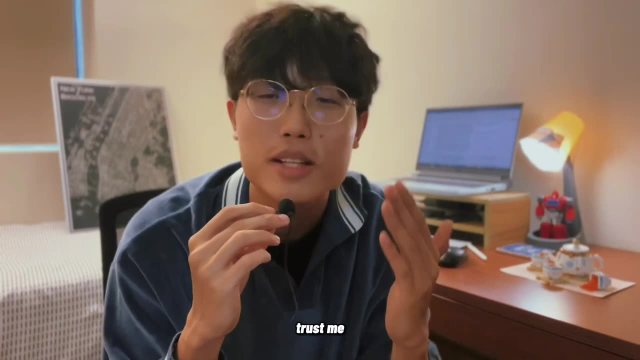 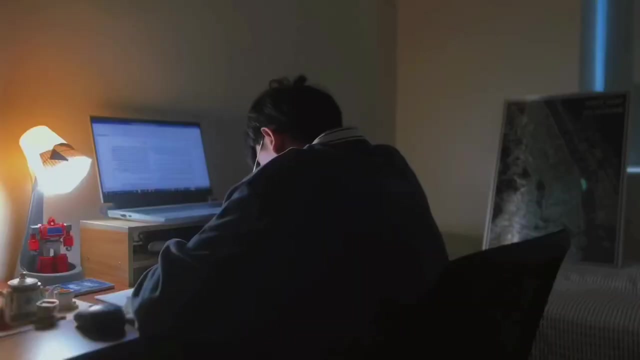 will not lose your momentum. Just the thought and action of wanting and actually squeezing time to do even just one question will go a very, very long way. Trust me, everything is about momentum And preferably, Once you have generated an unstoppable momentum, the next stage will become much easier and 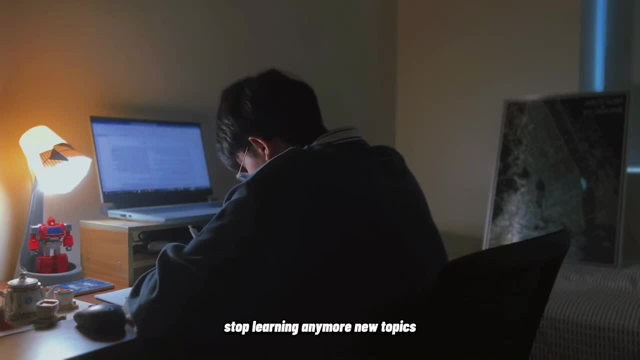 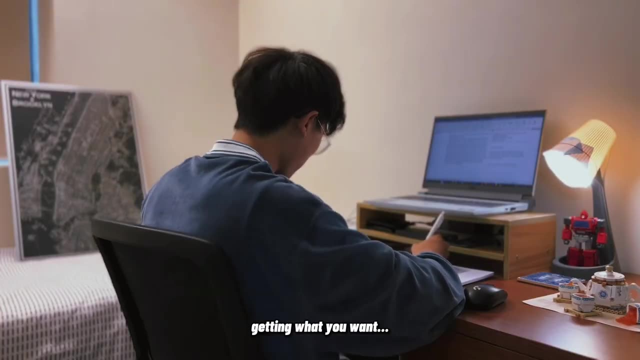 dare I say, more enjoyable because we can finally stop learning anymore new topics because it's exam season. In this stage, it is all about doing things that will maximise getting what you want- results, And the best way to do this is to simulate the actual exams over and over again until 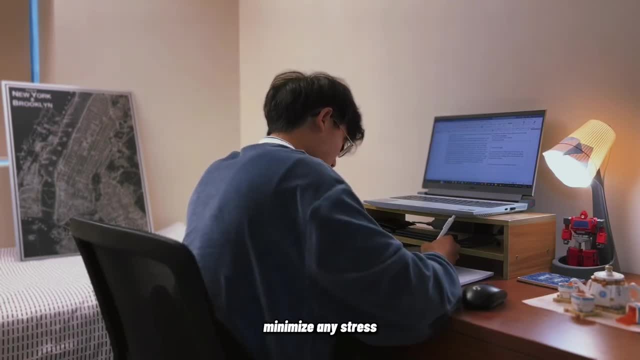 it becomes second nature to us. This can greatly minimise any stress and uncertainty, as you will be less likely to be caught off guard during the actual exams, As you will have known the format of the different exam papers. The closer you simulate exam conditions, the higher the chance that you will feel more. 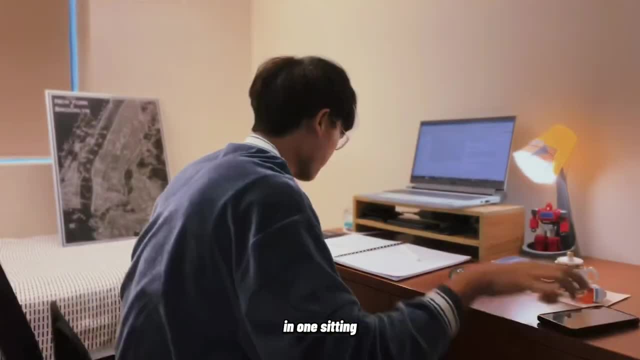 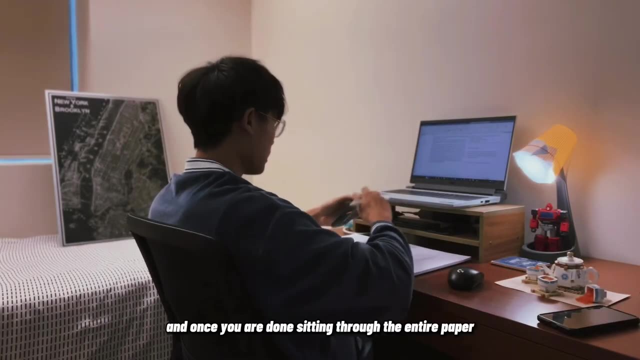 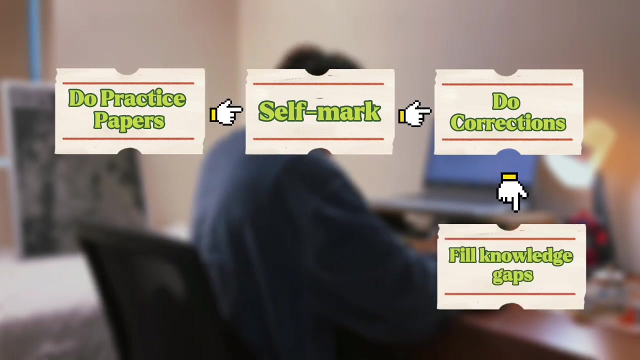 rehearsed. This means sitting through your practice papers in one sitting, under timed conditions, in a quiet environment without any music or distractions, And once you are done sitting through the entire paper, can you then start to check the answer key self-mark: do corrections? fill in your knowledge of content. gaps record: